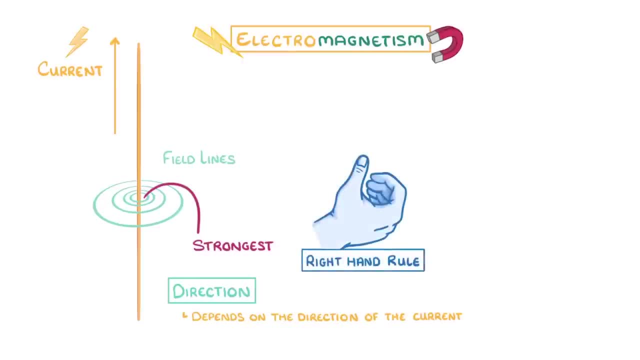 If you take your right hand, curl it into a fist and point your thumb in the direction that the current's flowing, then the direction that your fingers are curling in tells you the direction of the magnetic field. So for our wire, in which the current is going upwards, 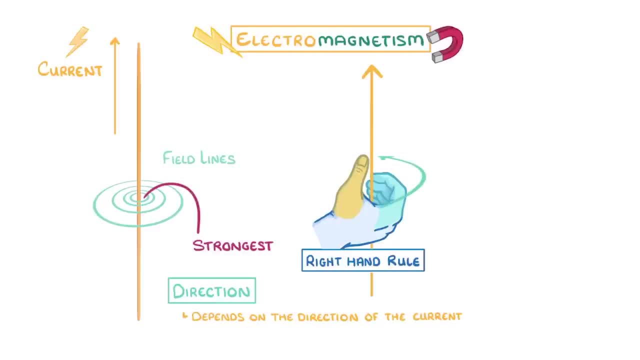 the magnetic field would be going anticlockwise, And so we would mark each of our concentric circles with little arrows in the middle. However, if we had another wire with the current going in the opposite direction, then, by using the right hand rule again with our hand upside down this time, we'd see that 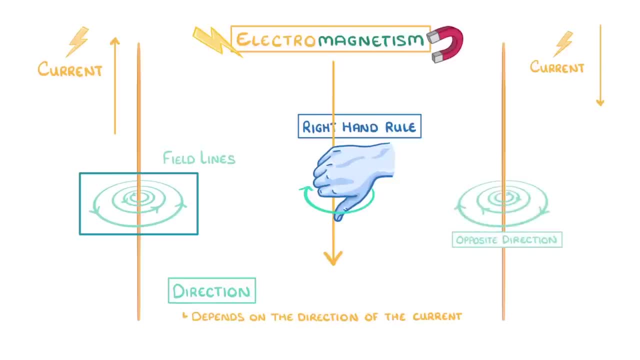 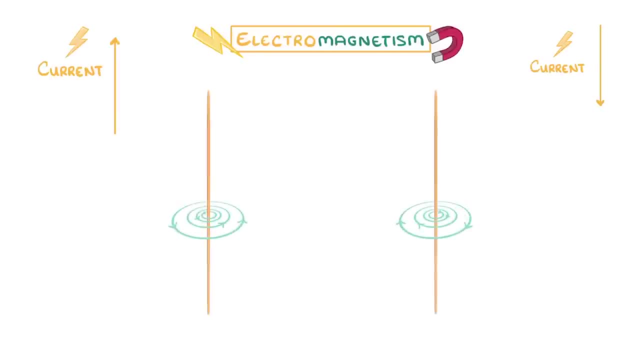 the magnetic field is now travelling in the opposite direction. To make things a bit trickier, let's now imagine that, instead of two separate straight wires, we instead joined them together so that we had a single flat, circular coil, With the current flowing in through the bottom left and out through the right. 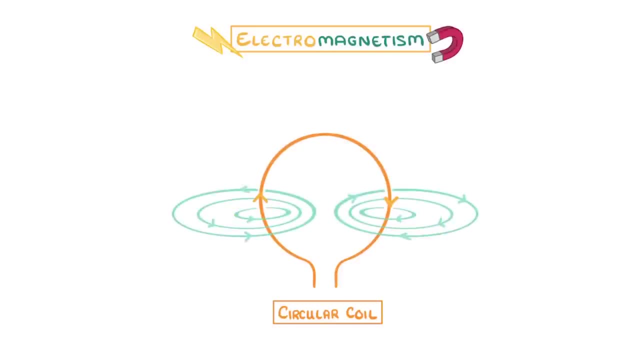 As the magnetic fields of the two sides of our coil interact, the magnetic fields, which were concentric circles, will now get stretched out and form ellipses, And as the magnetic fields combine, they'll form a single magnetic field which runs straight through the centre of the coil, Which, if we were to look at it from above, would look. 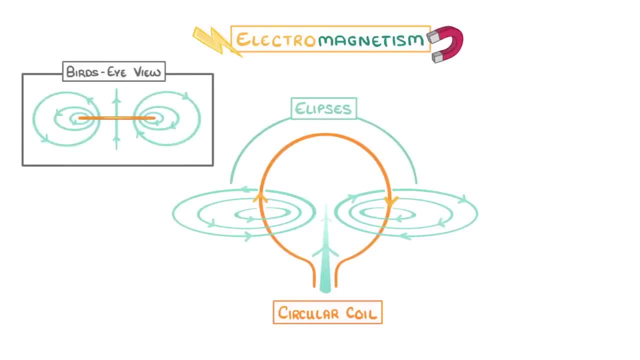 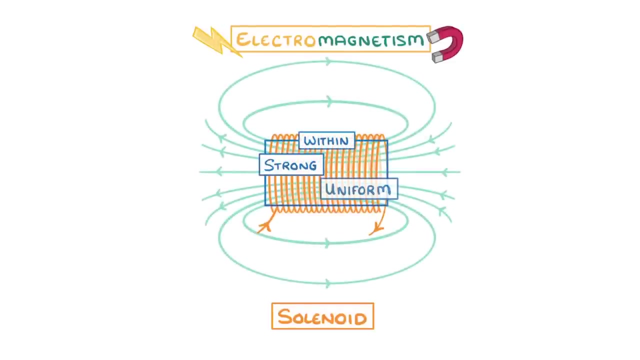 like this. If we now add lots more turns to our coil, all next to each other in one long piece of wire, we make something called a solenoid And, importantly, the magnetic field within a solenoid is strong and uniform. 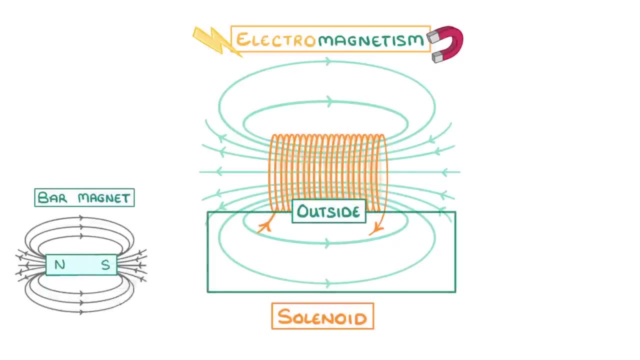 Outside the coil, the field is just like the one we'd find around a bar magnet. And just like a bar magnet, where the field lines come out is the north pole and where they point in is the south pole. So we've effectively used electricity to create a magnet, And so we call it an electromagnet. 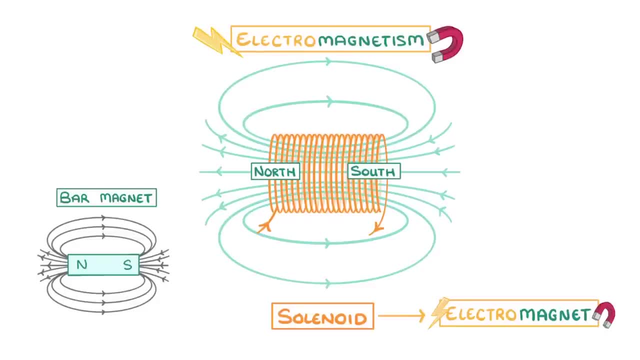 One of the useful things about electromagnets is that they're only magnetic for as long as we keep the current flowing through the wire. As soon as we turn off the power source, the magnetic field disappears, And when we turn it back on, it comes back As well as. 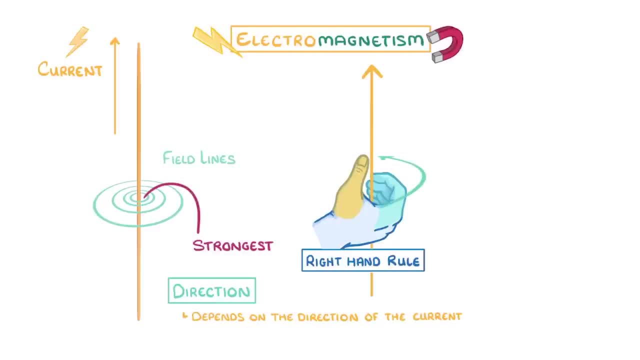 the magnetic field would be going anticlockwise, And so we would mark each of our concentric circles with little arrows in the middle. However, if we had another wire with the current going in the opposite direction, then, by using the right hand rule again with our hand upside down this time, we'd see that 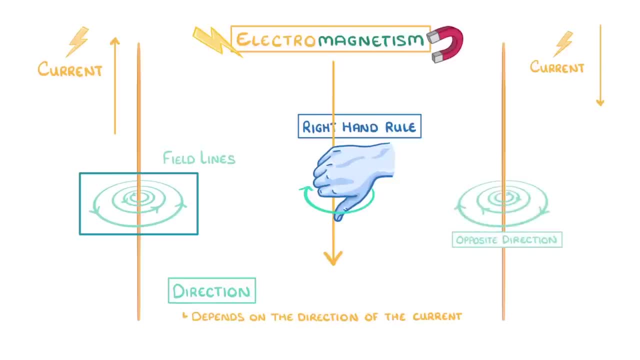 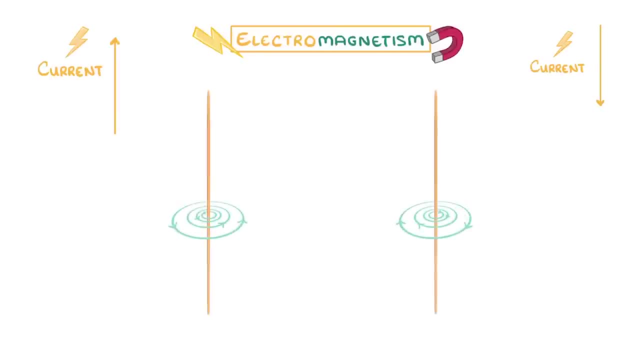 the magnetic field is now travelling in the opposite direction. To make things a bit trickier, let's now imagine that, instead of two separate straight wires, we instead joined them together so that we had a single flat, circular coil, With the current flowing in through the bottom left and out through the right. 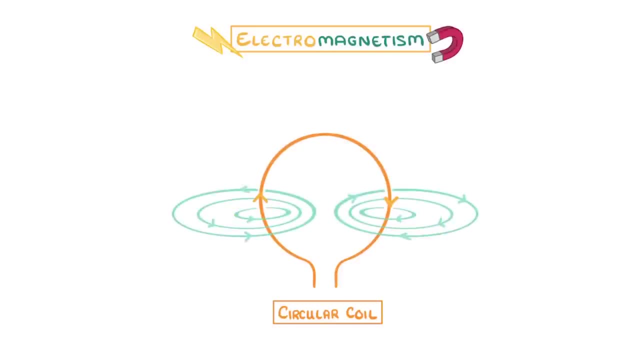 As the magnetic fields of the two sides of our coil interact, the magnetic fields, which were concentric circles, will now get stretched out and form ellipses, And as the magnetic fields combine, they'll form a single magnetic field which runs straight through the centre of the coil, Which, if we were to look at it from above, would look. 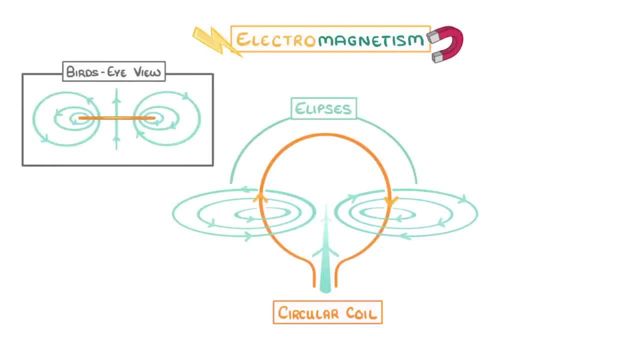 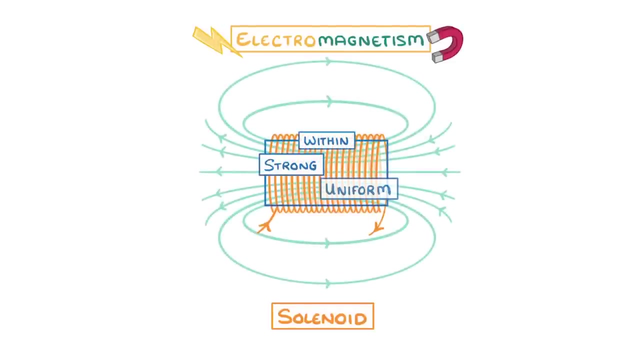 like this. If we now add lots more turns to our coil, all next to each other in one long piece of wire, we make something called a solenoid And, importantly, the magnetic field within a solenoid is strong and uniform. 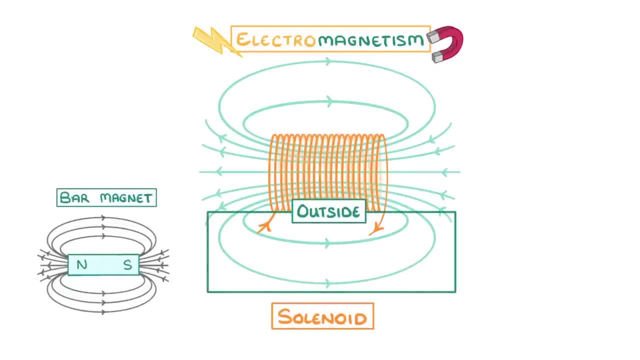 Outside the coil, the field is just like the one we'd find around a bar magnet. And just like a bar magnet, where the field lines come out is the north pole and where they point in is the south pole. So we've effectively used electricity to create a magnet, And so we call it an electromagnet. 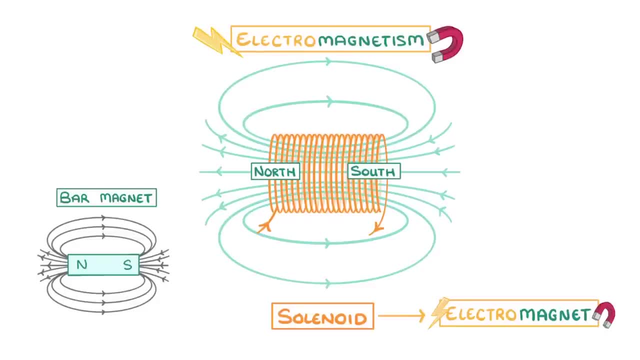 One of the useful things about electromagnets is that they're only magnetic for as long as we keep the current flowing through the wire. As soon as we turn off the power source, the magnetic field disappears, And when we turn it back on, it comes back As well as. 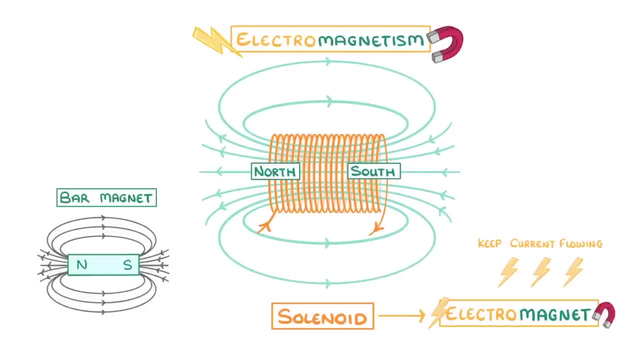 being able to turn it on and off, the magnetic field disappears And when we turn it back on, it comes back. And as soon as we turn it back on and off, we can also reverse the direction of the magnetic field by reversing the direction in which our current is flowing.